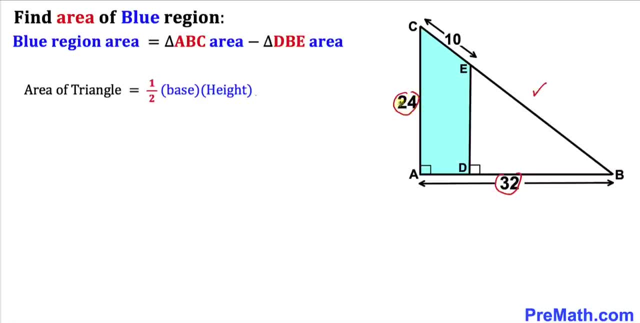 32 and our height is 24, so we can easily calculate the area of this triangle ABC. However, for this smaller triangle, DBE, we don't know the base and the height of this triangle. Let me go ahead and call its base as X and Y as its height, and now we are going to calculate the value of X and Y. 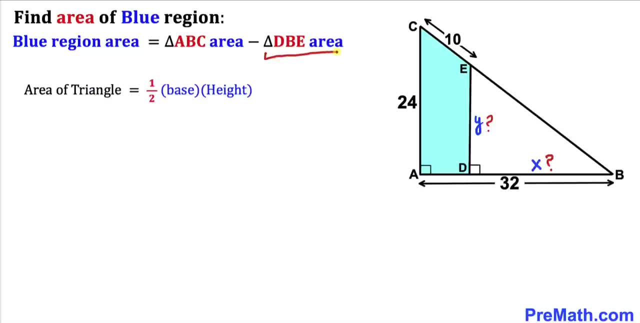 before we calculate the area of this triangle DBE, and here's our next step, Let's focus on this big triangle ABC. and we know that this is a right triangle, so therefore we are going to use the Pythagorean theorem in order to calculate its side BC. 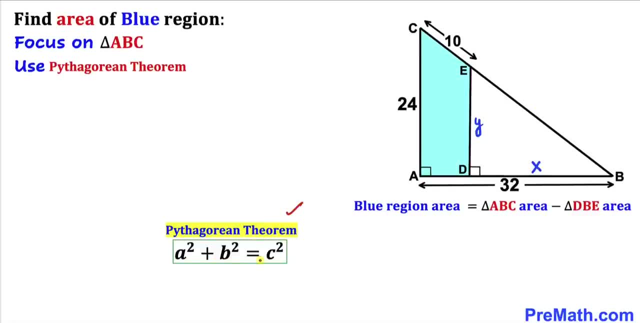 And now let's recall the Pythagorean theorem: A square plus B square equal to C square, In our case our this longest leg, I'm going to call this side C, I'm going to call this side A and this side B. So let's go ahead and fill in the blanks in this Pythagorean formula. A, in our case, is 32, so this: 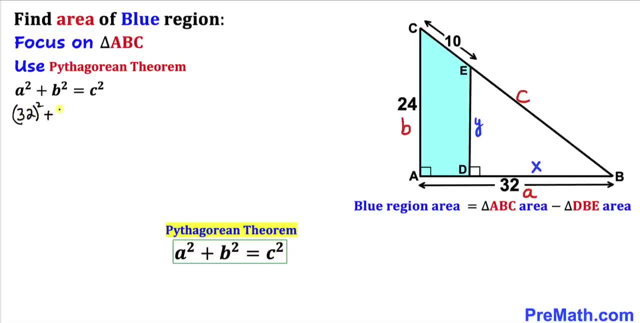 is going to become 32 square plus B is 24 square equal to C square. Let's go ahead and simplify: 32 square is 1024 plus the next square is 576, equal to C square. If we add both of them, C square equals to 1600.. Let's go ahead and undo this square on both side, so our C 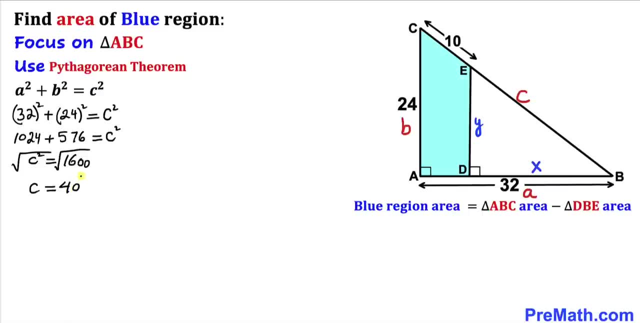 value is going to be positive 40 and we know that our side C, this high part in use, is same as the previous area. So therefore I can call length: BC equals to 44 Units. So therefore our this whole length, B, a, C, turns out to be 40 and we know that our this length. 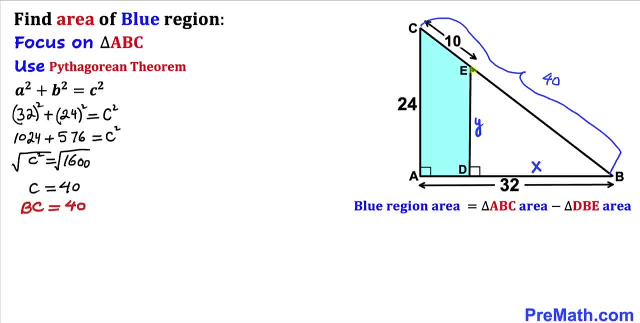 CE is 10 units. Oh, therefore, our this length EB is going to be 40 minus 10 is going to be 30 Units. So, therefore, this length EB turns out to be 30 units. Now let me show you an alternative method to this Pythagorean theorem. and we wanted to calculate this hypotenuse BC. 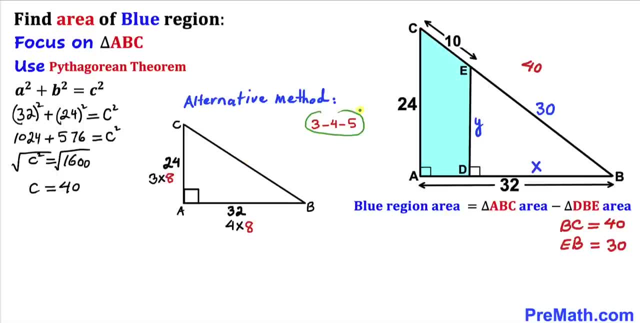 and now let's recall 3,, 4, 5 triplets. In other words, this 24 could be written as 3 times 8 and this 32 could be written as 4 times 8, and since this is a 3,, 4, 5 special triangle, so its longest leg could be written as 5. 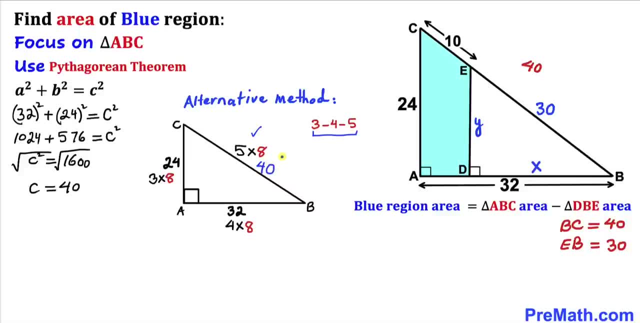 times 8, which is equal to 40 units. So therefore our hypotenuse turns out to be 40 units. Now we can see that these two angles are right angles, so therefore these two lines are going to be parallel. Then we conclude that this big triangle 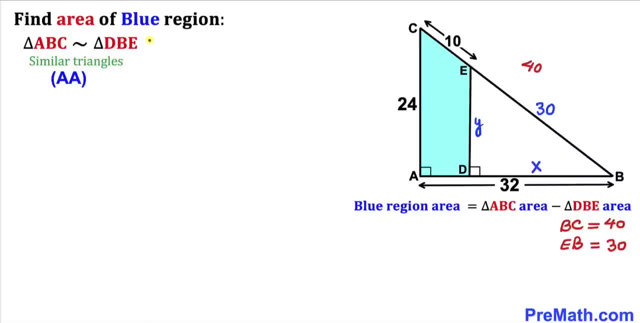 ABC is similar to this special triangle, smaller triangle, DBE, According to angle angle similarity theorem, since we can see that these are 90 degree angles, this is our angle in common and these are our two corresponding angles. So therefore, we are going to have proportions. so let's. 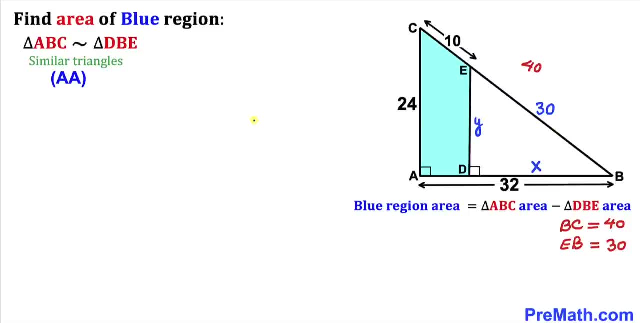 focus on these two triangles. We can have a ratio. we can write X divided by 30.. Let me go ahead and write down: X divided by 30 equals to this length: 32 divided by 40. So this is going to be 32. 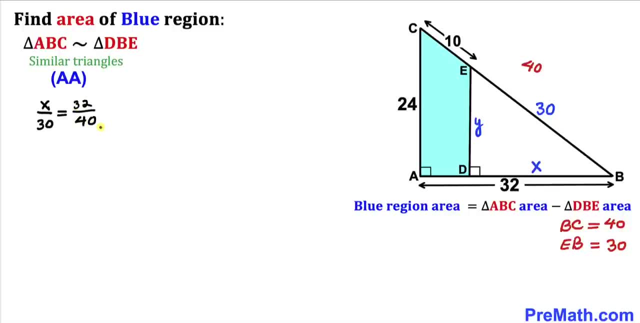 divided by 40. Now let's go ahead and multiply both sides by 30 to isolate X. We can see this: 30 and 30 is gone, so our X value turns out to be 24 units. so therefore our log length DB turns out to be 24 units, which is the 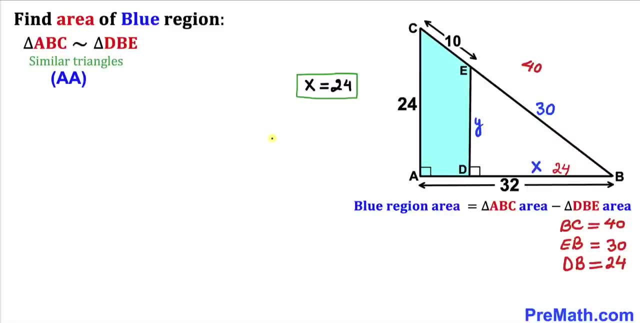 same as X value. Now let's focus on another ratio: Y divided by X. Let me go ahead and write down: Y divided by x equals to 24 divided by 32.. Let me go ahead and write down 24 divided by 32.. And we know our x values are 24 divided by 32.. 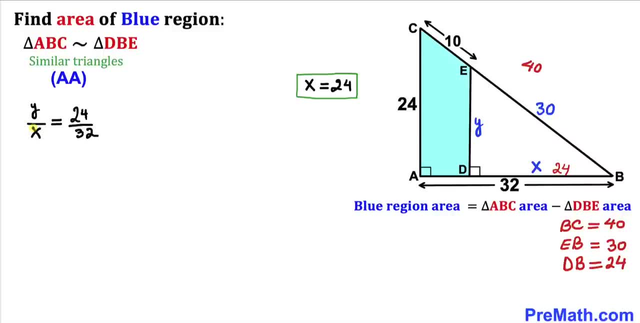 Let me go ahead and write down 24 divided by 32, and we can see that these two angles areist Neviks and one isат. x value is 24.. So I'm going to replace this x by 24.. So therefore, I can write y divided by 24.